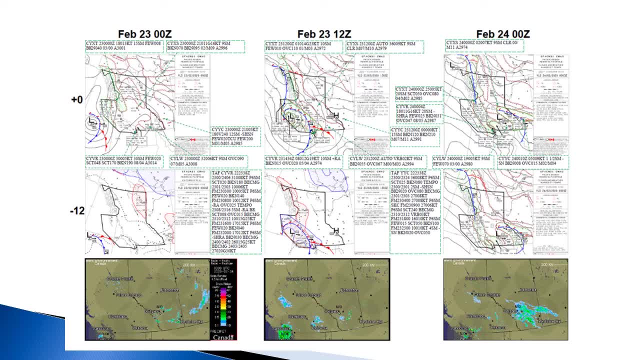 in color. I can get that done at Staples or a printing shot, And it's probably easier to follow along if you do that. So here's how I laid it down. So on February 23rd I downloaded a bunch of GFAs, METARs and TAFs. 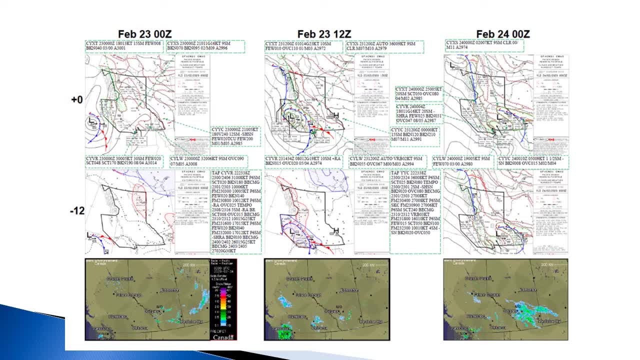 for different regions. This one is for British Columbia. I also downloaded a weather radar shot that we can discuss as well And you can see in the top. So these Were taken at midnight Zulu. So the top one midnight Zulu and then the one at 12 Zulu is 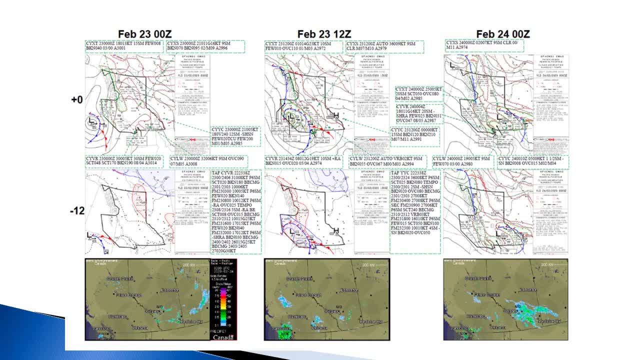 the subsequent clouds and weather: GFA. And then the one at midnight Zulu on the 24th- the 24 hours later is the one that was forecast at that time, However, what I did for the icing and turbulence chart, so that's the bottom one, the bottom GFA. 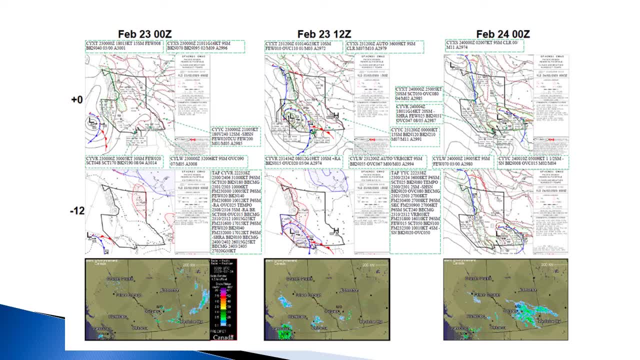 is. I took it for the same time, So the one from the top and the bottom are at the same time. However, it was the forecast from 12 hours earlier, So you can compare what they were forecasting 12 hours earlier with what they decided to forecast for what was going to happen. 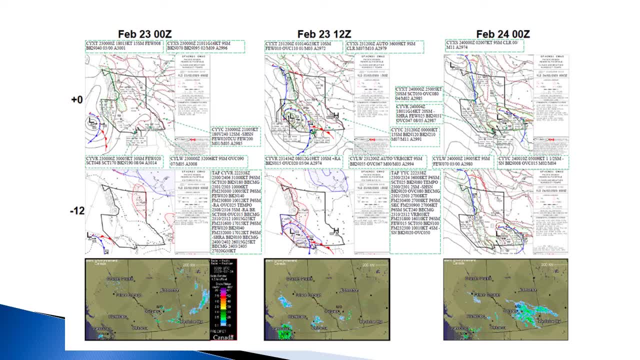 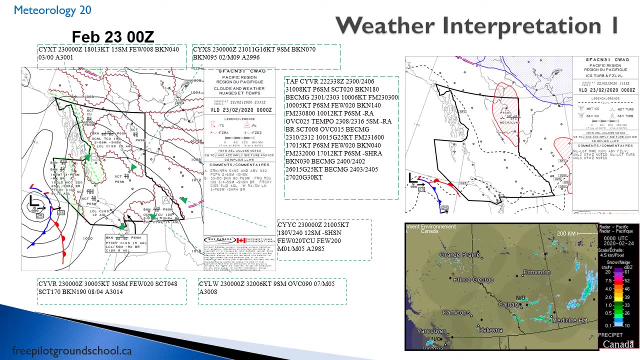 within the next half an hour, let's just say So. the one where the validity period and the effective time are the same. So we're going to go through these. I'm going to zoom in a bit on the different ones and then we'll just work our way through it. So let's begin by looking at the GFA. 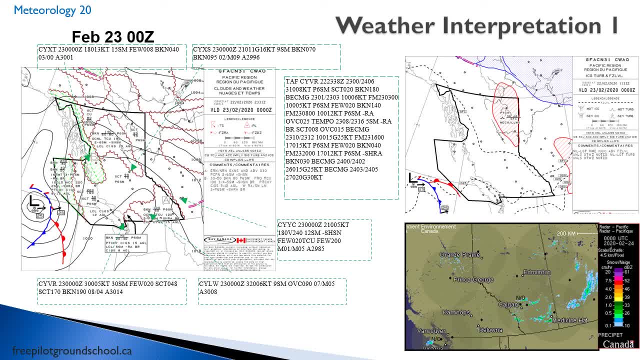 from the 23rd at midnight Zulu. So the clouds and weather are going to be on the left and on the right. is the clouds or, sorry, the icing, turbulence and freezing level? GFA taken for the same validity period but issued 12 hours earlier, on the 22nd, at 12 Zulu. 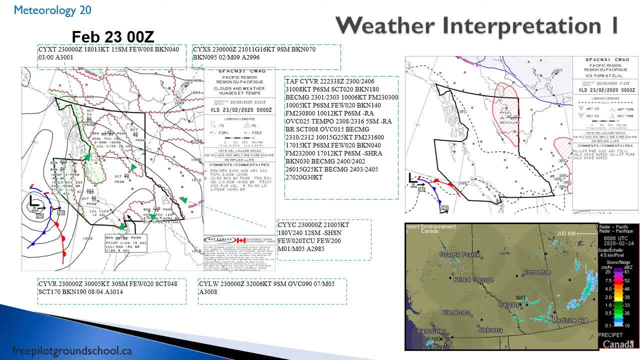 So let's begin. This is British Columbia. Hopefully you're somewhat familiar with British Columbia. I did put arrows in where the actual weather stations are, Should you not know where, let's say, Terrace is or Prince George? hopefully that'll become a bit clearer to you. 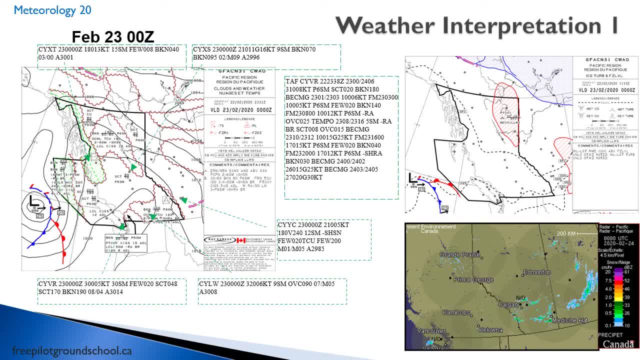 So let's begin by looking at the GFA portion. So if we look on the left side, we see this frontal depression here. Here's this low east at 25 knots the lowest, as is this occlusion right here, or trowel, we have a. 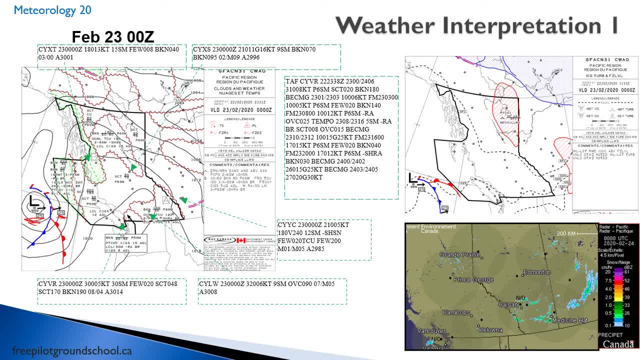 cold front catching up to a warm front. so if we were to look at this right here, okay, so just try to think about how this would look like from the side. okay, so we would have a warm front. okay, and then I'm gonna draw the ground here. this is: 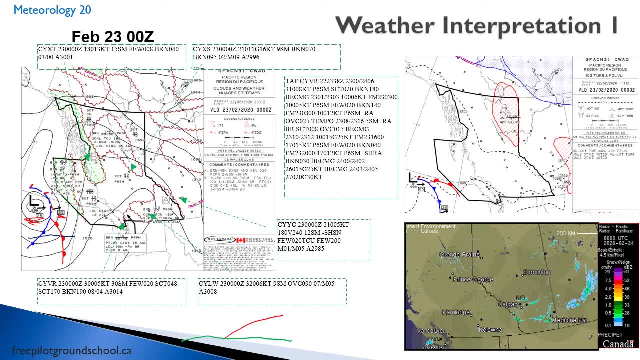 just how it looks like. and then here will be the, the cold front. okay, this would be warm air, right here, warm air. and then this would be cool air. we'll just call it cool. then this will be cold air right over here. okay, so the cold air. 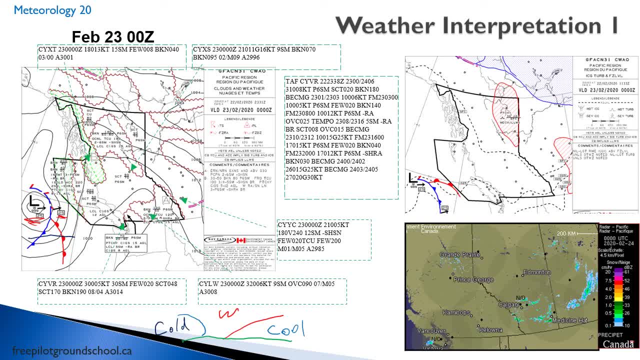 is catching up to the warm air, and so that's how this would look like. if we draw this cross-section right here, you can notice the ISO bars are quite close together, so you're gonna have strong winds. and if we look at the GFA here in this region right here- okay, we could take a look- it says it's broken. 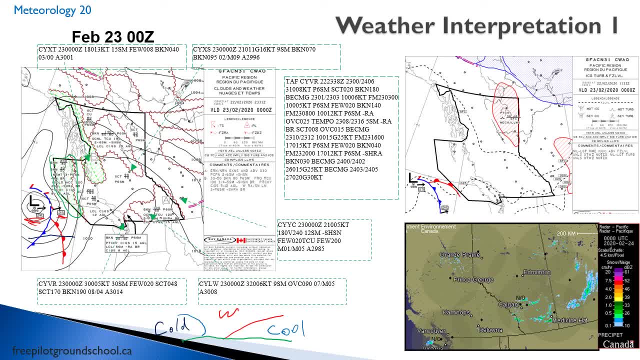 with the bases at 8,000 feet, tops at 20,000- remember it's ASL- and then there's a second layer, broken at 2,000, tops of 4,000. there's intermittent visibilities, three to six statute miles in light, rain and mist, isolated, alto. 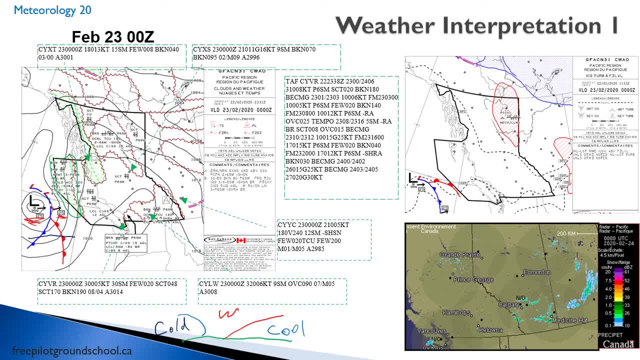 cumulus castellanus tops at 22,000. so because it's after the cloud, that means it's the top two statute miles in light, rain, showers and mist. there's patchy ceilings: 800 to 1,500 feet AGL. now let's move over in this region, right here we'll do purple, so we haven't. 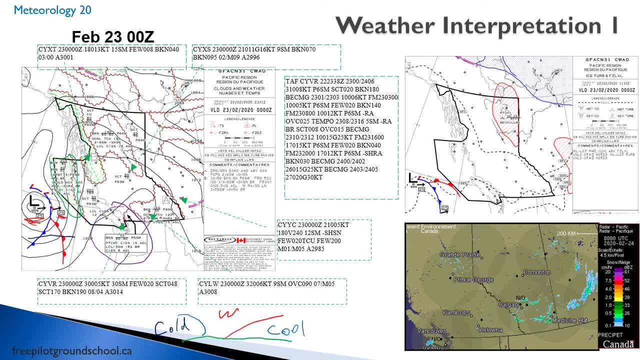 seen purple. yeah, so this region right here is Vancouver area. it says it's broken. they're forecasting broken, with bases between two and four thousand feet, seven thousand feet of the tops, plus six statue miles- and patchy sealants: 1500 AGL local uh, five miles in light, rain and mist sealants at 800.. 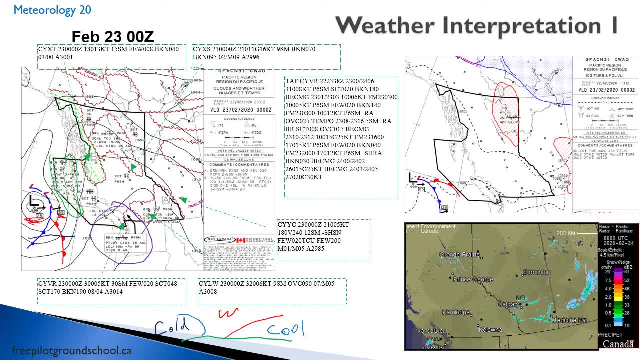 so let's compare that to what the actual METAR said. so this was what they were forecasting at midnight Zulu, so it came out half. it was released half an hour prior 23: 30 on the 22nd midnight Zulu. that's what they're forecasting, and then 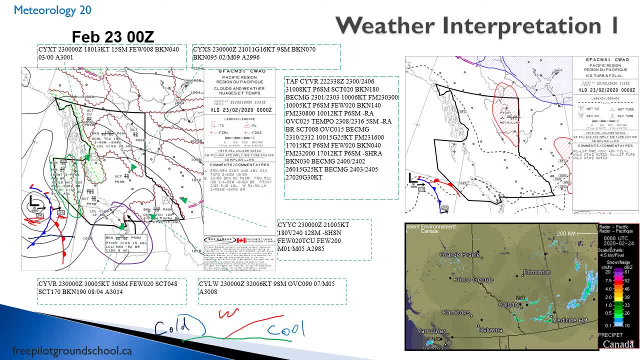 what was the actual weather in Vancouver? so if we take a look here, I'm 23 at midnight, Zulu Vancouver, winds 305 knots. so that makes sense, because look at the isobar, uh, they're pretty far apart, right here, 30 miles. few at 2,000 feet, scattered at 4,800. scattered at 17,000, broken at 19,000. temperature. 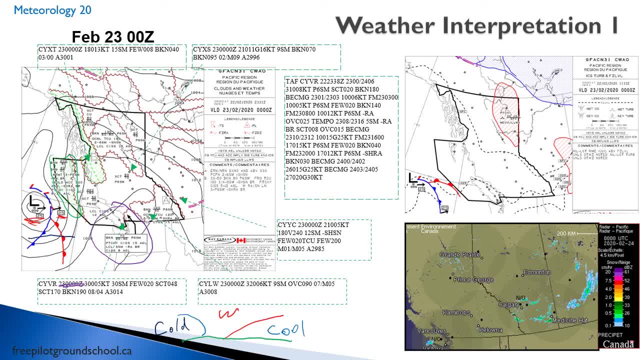 eight, two point four. altimeters: three zero one, four, so there's no ceiling there. but it said it was Apache ceiling, but they were forecasting that there was a broken layer between two thousand and four thousand. so in this case we would that would probably be this few, so it wasn't actually a ceiling. it ended up being better. 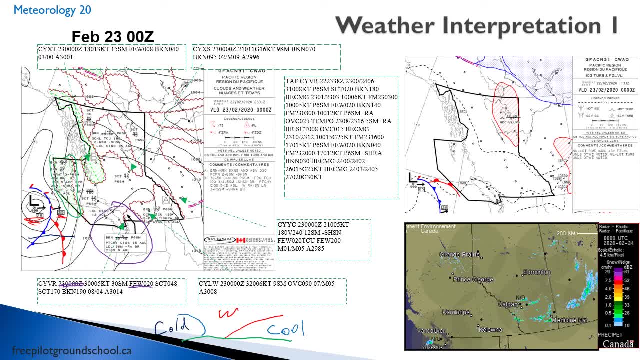 weather than what they were forecasting. if we look over here at Kelowna- uh, we look, and uh, your Kelowna would be like right there, I think that's Kelowna right there. so if we look at this area right here- okay, so that area right there- uh, they're calling broken bases at six thousand. 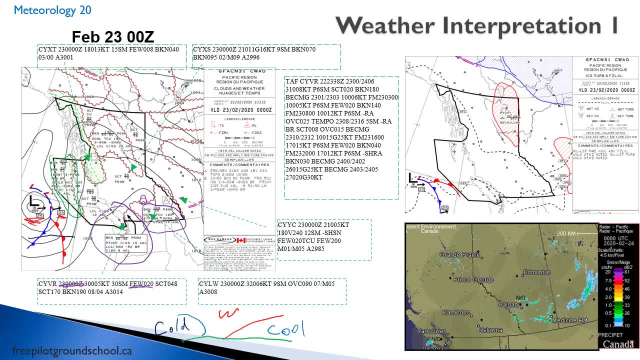 tops to ten thousand, uh, the towering cumulus, light rain showers, um so uh, the actual weather at that time, though, is light winds. nine statute miles overcast at 9 000 feet, so they're calling broken, uh, between six and ten thousand, so nine thousand feet. 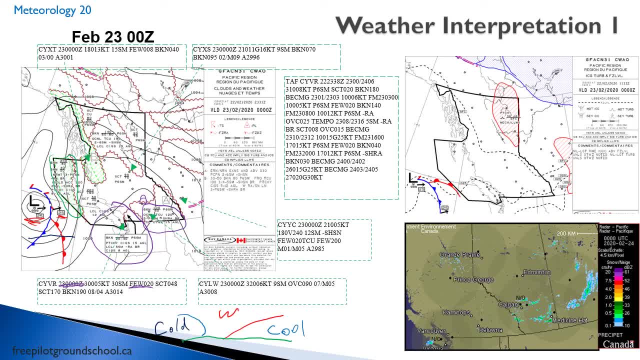 that's quite reasonable. there's also an A there, so let's look at what the A says. A remember on the comments over here. okay, so this is Eastern Northern sections and above three thousand feet precipitation: two to six, that two miles light snow showers mountains here. so they're just saying in this area, just be aware that it might be bad weather. 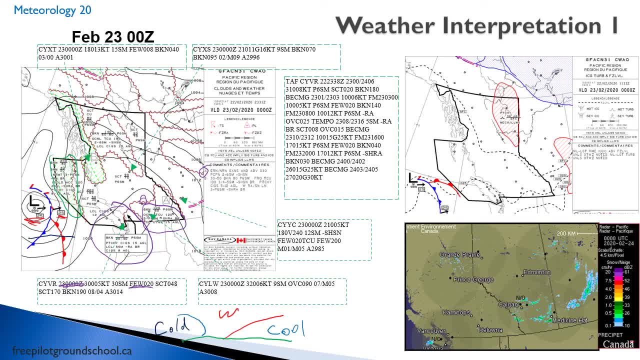 up up in higher areas in the mountains. let's move across here to calgary. okay, calgary, looks like it's pretty good weather here and uh, however, you can see here in calgary it's actually: uh, if we look at the metar over here, calgary, midnight zulu, we have light snow showers. 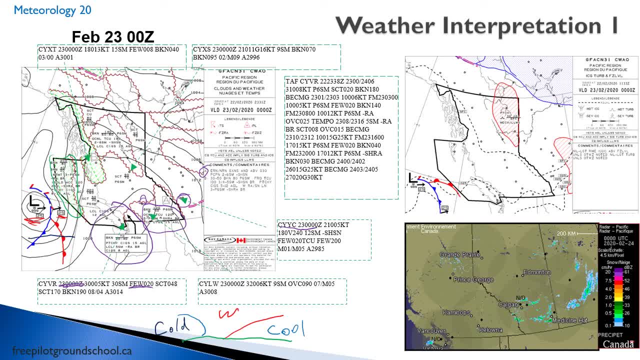 few at 2 000 feet. so, even though calgary, uh, looks like it's clear right here, it appears that it has been influenced by this weather system. okay, see this weather system, which is this weather and colonna. so what that tells us is that this weather here, um, where they're saying that there's light, 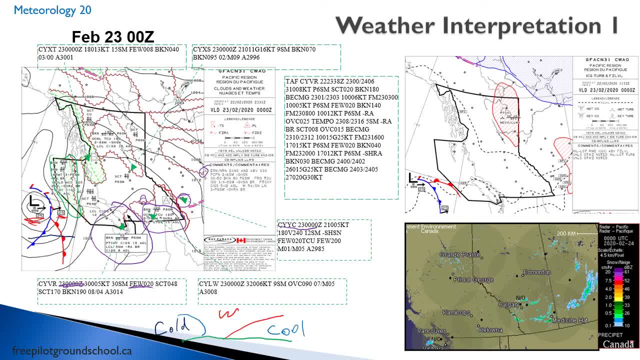 snow showers and mist feelings of 1500 feet and towering cumulus. so that's actually moved faster than they were forecasting. so that would be why colonna has better weather than it was forecast, because there's no snow showers in colonna and the ceilings are higher, so that whole cloud system is now over calgary actually moved faster than 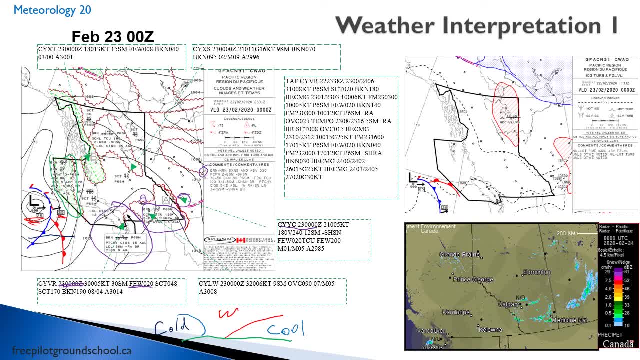 they were forecasting and colonna is kind of behind it now and colonna is in the clear. okay, let's move up north to, uh, prince george yxs up here. so if we look at the gfa in that area, uh, they're calling scattered at bases at seven thousand, tops at nine thousand. so it's. 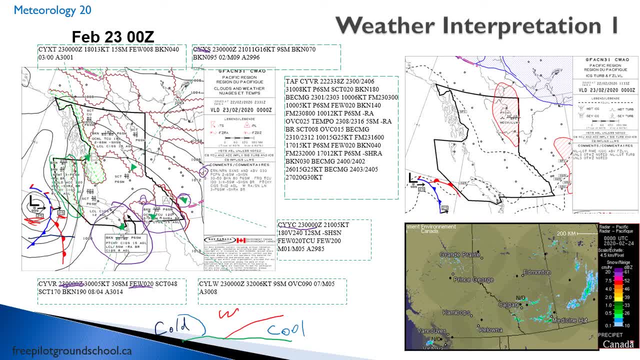 nice weather there, plus six statute miles visibility, and then, if we look up here, so it's gusty winds. uh, two ten eleven got sixteen nine statue miles, so that's better than six, and then broken at seven thousand feet. so that's pretty much exactly what they're forecasting. 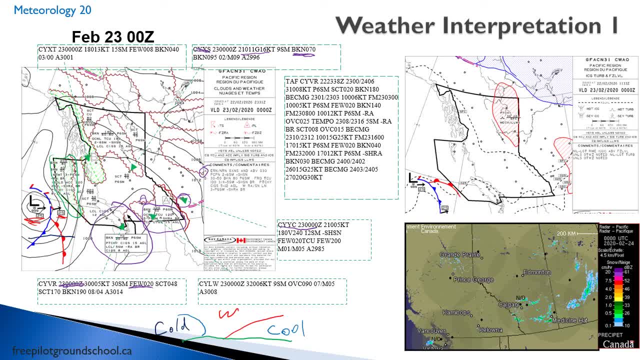 it's broken at seven thousand feet, don't mind you. that's agl, remember, and the uh, the uh. gfa says asl, but it's still uh, kind of within that same ballpark, so that, uh, that forecast looks reasonably good and then let's go order this and that's asn. eventually, that's only one fall. trouver lightning currently walked some hospital metaphor. 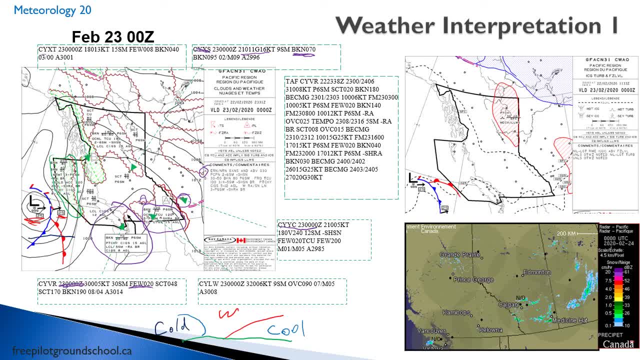 so that, uh, that forecast looks reasonably pretty good. and then let's go to the top here. uh, look at terrace bcyxt. it's on the pretty much on the coaster just inland of the coast, uh, the west coast of british columbia, and we look at b, so there's clouds and weather. 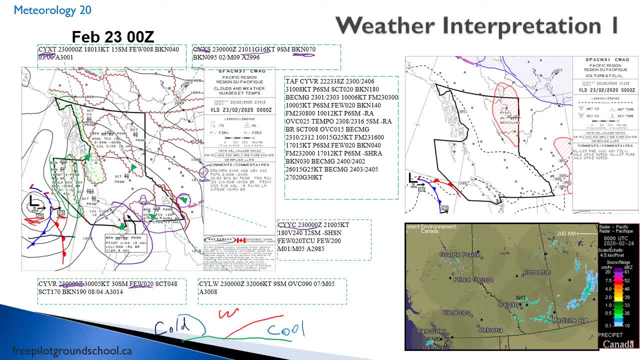 there. let's look at b, says to remember b over here. okay, and we'll look at that. so they're calling bases at three to five thousand feet, asl, broken tops at eight thousand plus six at your mouth, frequent towering cumulus tops at ten thousand feet, three quarters to five miles and light snow. 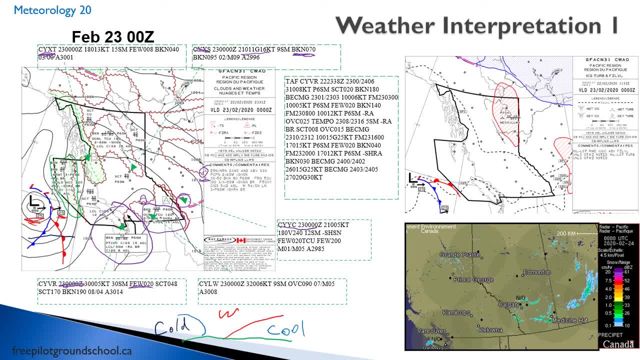 showers and mist, patchy ceilings, five to twelve hundred agl and uh, so that's kind of miserable there and uh, we look at it and here it actually says 50 miles few at 800, broken at 4 000.. so that's actually quite a bit different, so there could be a number of reasons for it. that system. 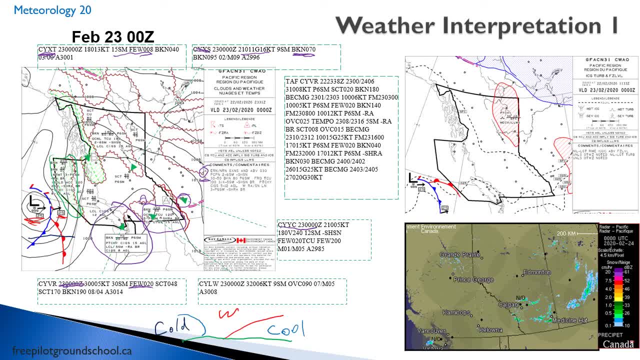 seems to be more typical of what you would see in prince george here than it does here. so my guess is this system may not have moved fast, as fast as they were anticipating, so it's not quite there yet, but we'll see what happens, uh, in 12 hours. so let's look on the right clouds and, uh, or sorry, uh. 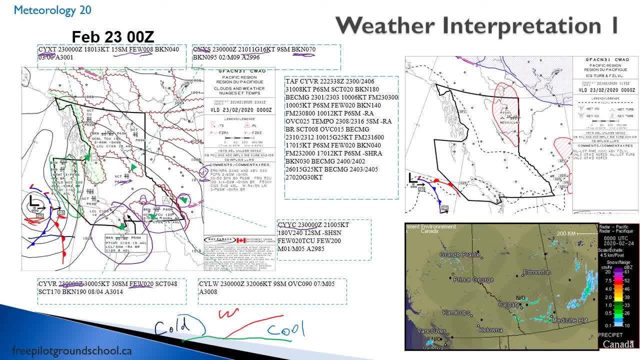 freezing level and turbulence: icing. freezing level and turbulence: gfa. so this is what they were forecasting: uh. on the right here i'll just underline it: this is what they were forecasting 12 hours earlier. so you can see, if we look here at this low and the uh, the. 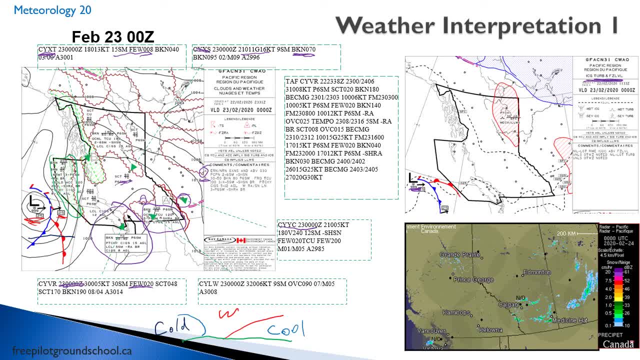 front. so 12 hours earlier they were forecasting that this front would be considerably, this frontal system here would be considerably more uh, rotated, so kind of it, rotated a bit quicker. and then by the time they got to the, the validity period of midnight, zulu, it was uh, it, it's kind of more steep. 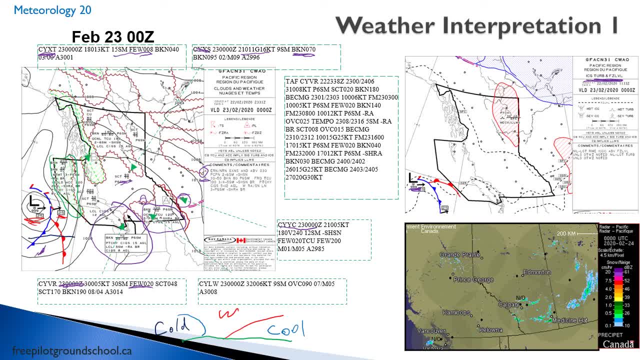 if you look here, notice how it's not, as it's more vertical here than- and it is on the uh icing gfa, but we can look over here. this time they were forecasting, if we look here. okay, so patchy. uh, they were looking at patchy. 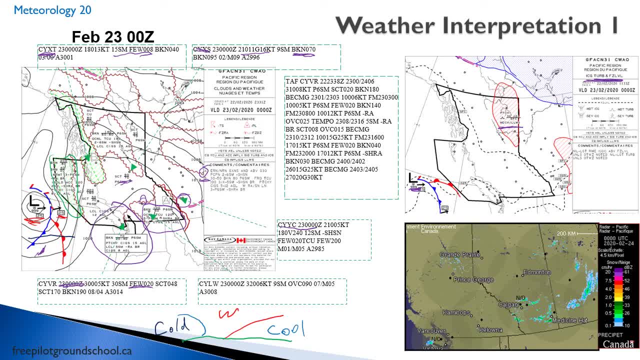 moderate turbulence from the surface to 3000 feet. agl. mechanical low-level wind that's caused by the winds. uh, so that would be. if we look at prince george, for example, remember, it's gusting 16 knots. it's in the mountains. it's going to cause quite a bit of. 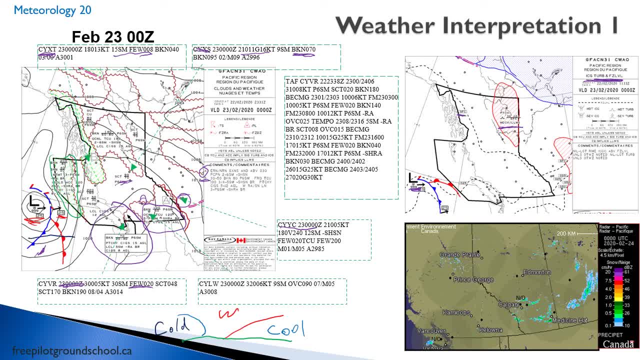 and uh. if we look at freezing levels here it's mostly at the surface. so along that line freezing levels will be there. that will happen at Myers capture point. it's going to have a high for what's going to be at the surface. let's look at the task over here for Vancouver. so i just gave one. 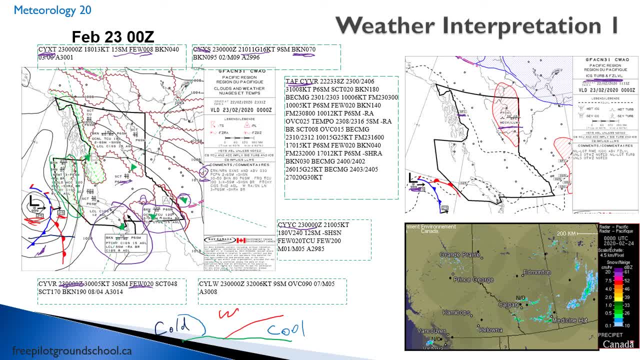 example. so between midnight and zero six zulu, they're calling three ten at eight knots, plus six miles, scattered at two thousand, broken at eighteen thousand. so that's pretty much what the metar over here uh indicated. so we'll see how that develops as the time progresses. 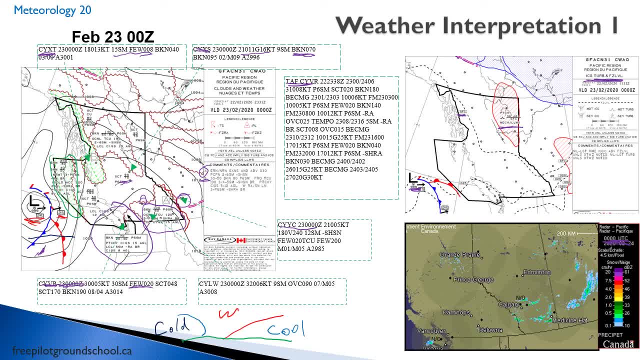 says 12 Zulu here, and so this covers just Vancouver, or, sorry, British Columbia area, lower British Columbia, and then also covers Alberta. but we won't pay attention to Alberta because it's kind of outside of the GFA region so we might not get the full clouds and weather. 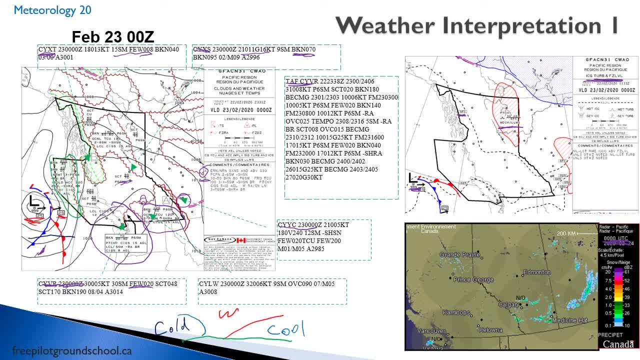 impact of the clouds and weather. so if we look at 12 Zulu, yeah, there's not much. there's a bit of precipitation right down here, okay, and that's basically what we see outside of Vancouver, but it's off the coast, but it's pretty much clear here. there's not, there's not too much, too much snow. 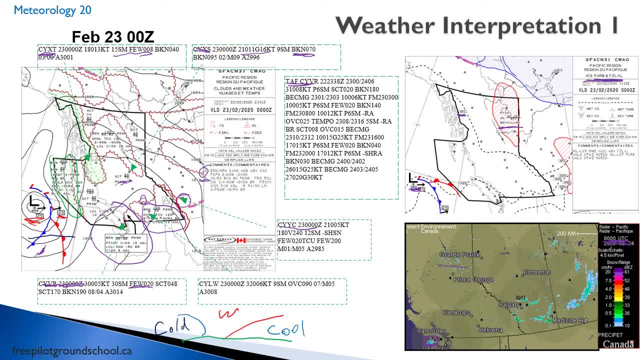 going on here a little bit up north of Prince George if we look up here, which makes sense with this weather up here, where it's just light snow showers but not really heavy returns, strong and strong precipitation. so let's move on to the next uh slide and see how this weather system has progressed. so here we are, 12 hours later, February. 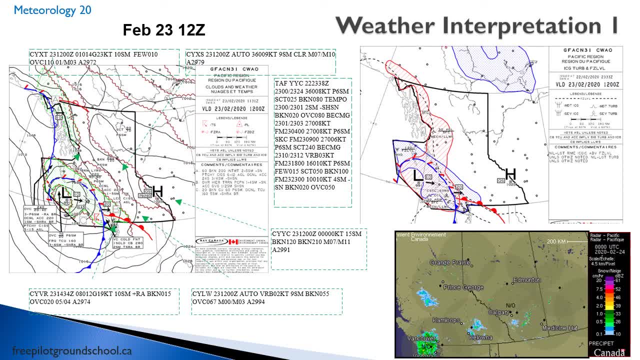 23rd, at 12 Zulu. this uh the clouds and weather. so this was issued at 11, 31, 12, 30. so this is they. they came up with this forecast for something that's going to happen in half an hour and lasting half an hour for another 12 hours. so now we can see that this frontal system is completely uh over. 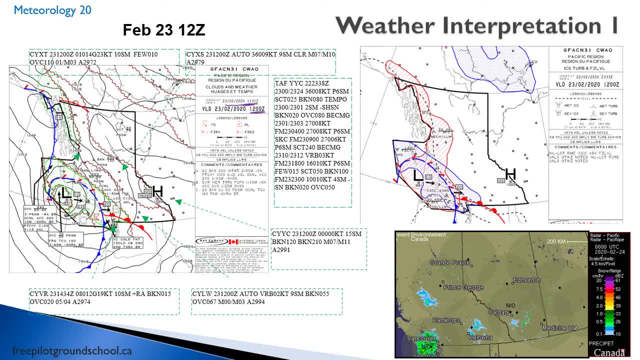 at this time- and this is really important to notice and remember here- how we said that this cold front is catching up to the warm front, and then we have this occlusion and you end up with just absolutely miserable weather. so let's look over. uh, we'll start on the left side here. uh, with 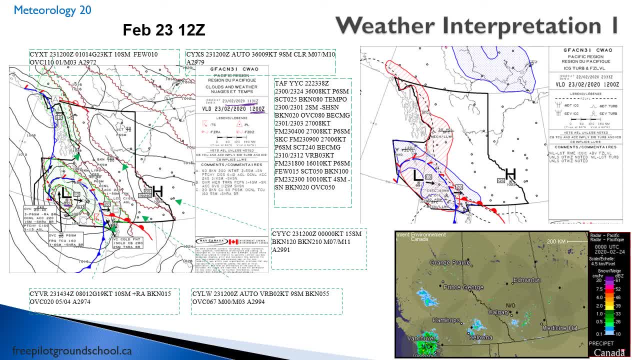 this low. the low pressure, I believe, is 991 hectopascals. the weather in that area, in the clouds and the weather area there is, uh, overcast. so if we look over here, okay, so look at this box here it's overcast, two to four thousand feet asl tops at twenty four thousand. so 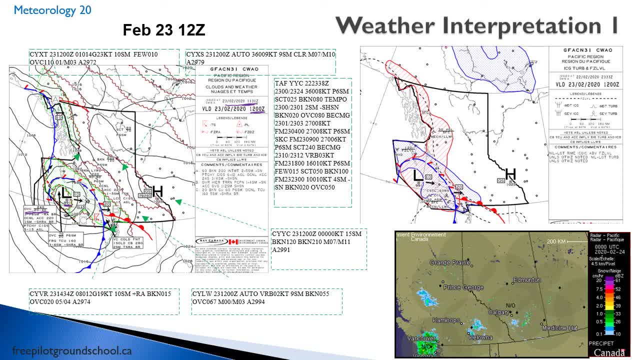 that's a solid layer of cloud that's pretty thick and uh the visibility: three miles in light rain, mist, occasional to females. castellanus topping at twenty two thousand one statue miles in light snow. uh, rain showers miss patchy ceilings. five to fifteen hundred feet, that's uh up here we should. 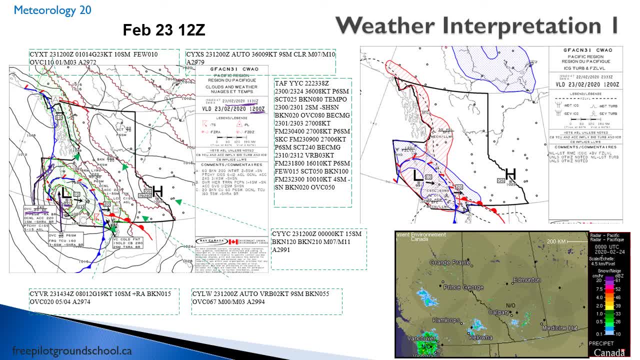 notice. so on the north coast of the queen charlotte's and then right here we'll look at this area. so I'm just going to circle this to make your life easy. uh, overcast at two thousand feet. tops at seven thousand plus six statue miles. frequent, uh, tyrant cumulus. tops at sixteen thousand feet. three. 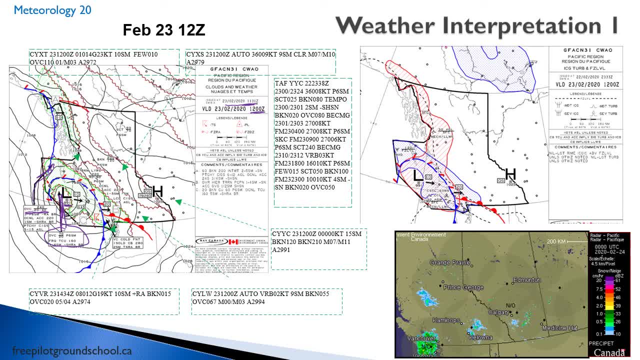 to six statue miles: light, rain, showers and mist. so again, like I said, occlusion, miserable weather. you have strong winds, you have towering cumulus, so, and you could get thunderstorms potentially. let's say this was the summer. you get thunderstorms, but then you also have rain showers and mists. so 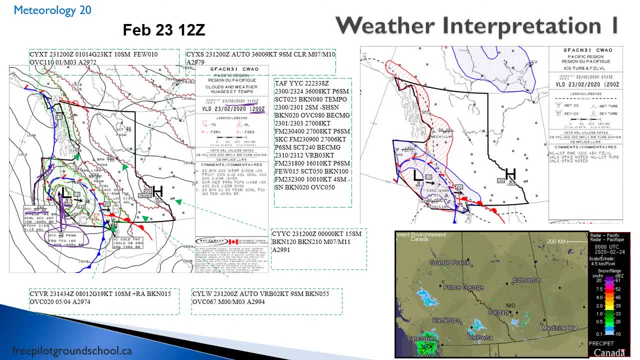 uh, kind of warm front weather, absolutely miserable. now let's look here. let's look at this is vancouver what the actual weather is in vancouver, and we can see vancouver. if we just follow the arrows, going to be right there. so this is right after the warm front went through. the wind: zero eight. 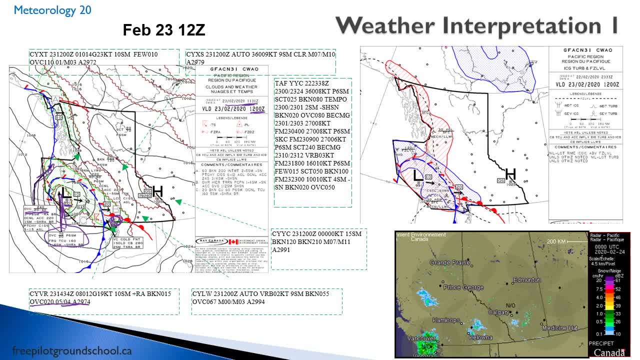 zero twelve gusts, nineteen so dusty winds, ten miles in heavy rain, broken fifteen hundred feet and overcast at two thousand feet. so that, uh, that is quite miserable. they're also saying, they're also forecasting here. if we look right here, in the vicinity of the cold front isolating cumulus, tops at twenty eight thousand. 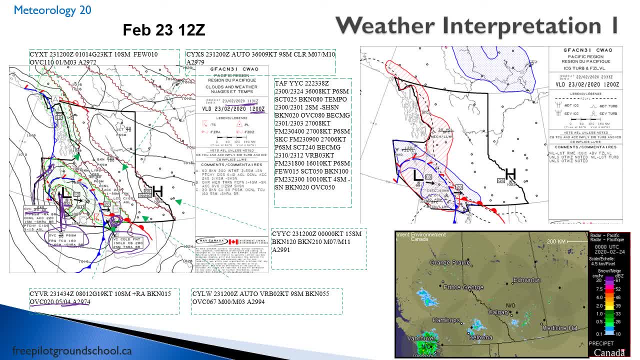 two miles in thunderstorms and mist- absolutely miserable day. however, if we start looking at the clouds and weather for Kelowna, which I believe is here, Kelowna actually might be here. I can't quite. it might be that the farther one to the north, but if we look at the, 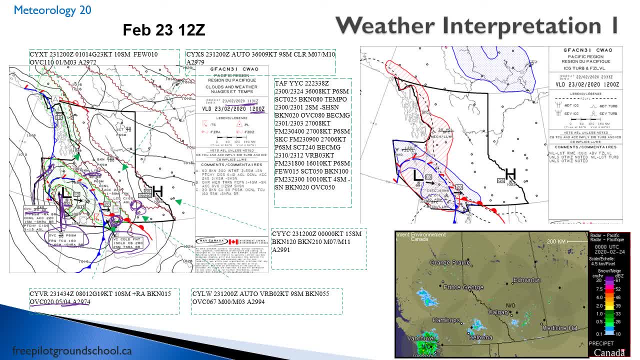 this weather here, where it says so, it's talking about uh, broken layers, uh, at bases, four thousand to six thousand, plus six statue miles with the occasional ultra cumulus castle, and compare that to the metar with Kelowna: right here we have light winds, broken at fifty. 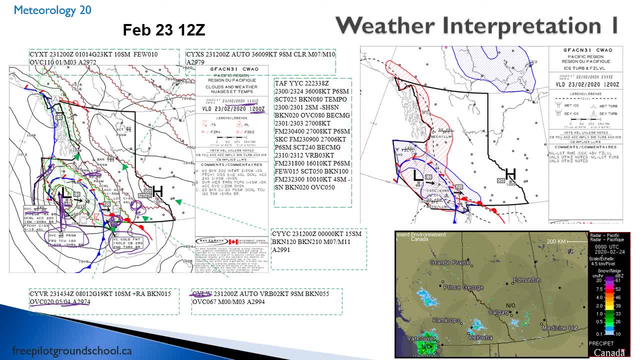 five hundred feet agl above ground level. so Kelowna, I think, is about fifteen hundred feet. so they go seven thousand feet, so that makes sense. um it, the the ceiling is about what was cast on the gfa and uh. temperature zero minus uh, and the two point is minus three. we'll look at. 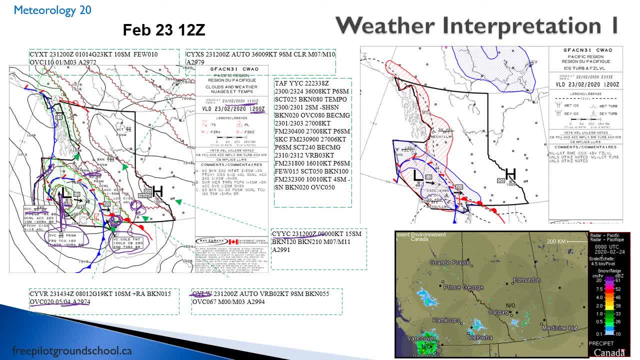 Calgary. now Calgary is outside of the um of this region, so you won't, they won't display all the weather that's there, mostly blank, but it is uh, fifteen miles broken at twelve thousand feet, which is quite nice. let's go north. Prince George is here. it's kind of central BC they're calling. 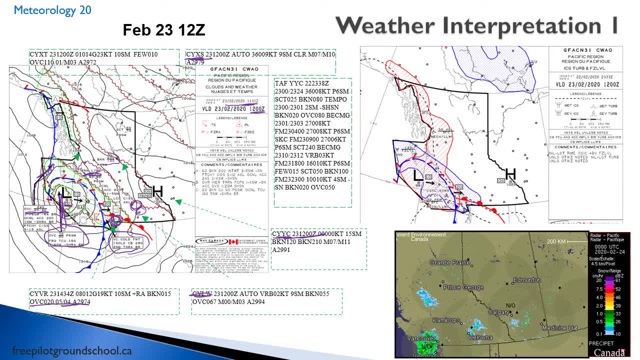 on, uh on this right here there. so it's clear in Prince George and uh the. but they're forecasting bases at twelve thousand, tops at twenty thousand. so, uh, something interesting here, because this is an auto station. if it's an auto clear, sometimes it will come back as clear instead of sky clear. 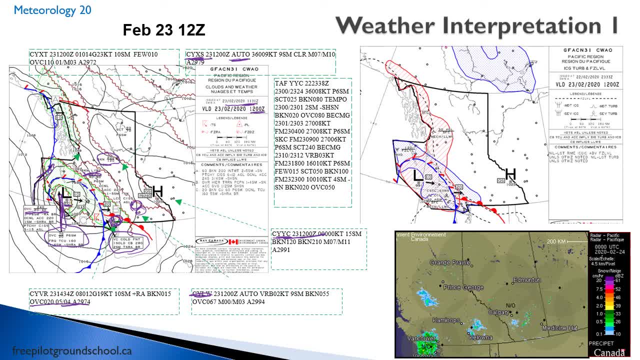 so when you see skc, the actual sky is clear. the clr is just the auto station, doesn't detect any, any ceiling. it could still be sealed way high up, but it's not going to detect anything. if we go to terrace on the coast, okay, it's gusty winds to 23 knots. notice how close these. 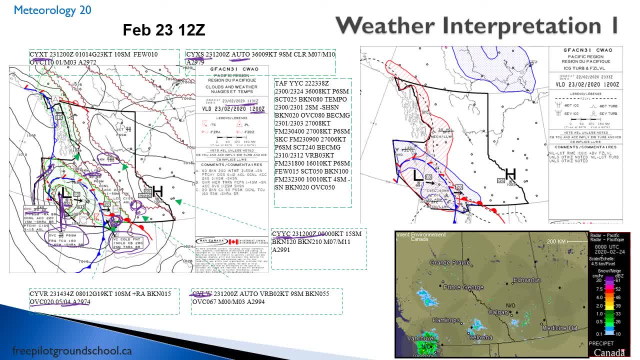 isobars are together, okay, and when zero, one zero at 14, gusts 23, so um that that's caused by the strong uh pressure gradient there, uh here, remember, this is an upper cold front, right here it's a very low markings, okay, and then an upper warm front- okay, so we'll just draw it out. so 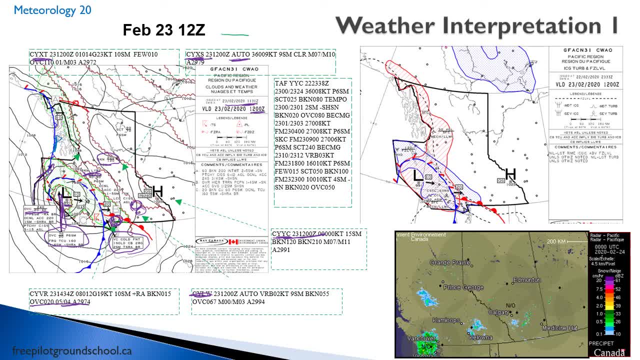 remember, let's say we have the ground. I'm just going to draw it out up top here. we have the ground and then we have an upper- um, warm front might be like so. so an upper warm front would look like so it's a a layer of, uh, warm air and uh, uh and uh. 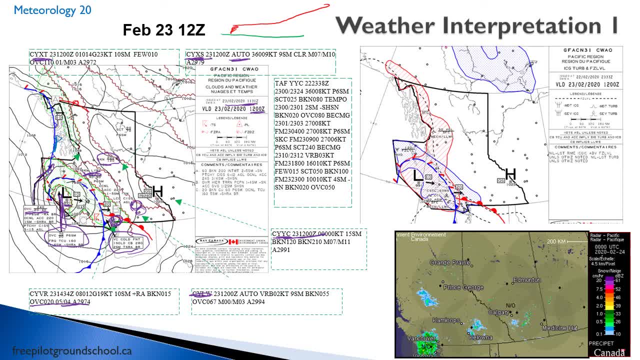 the uh and then the front kind of sits on top of uh, of the layer of uh of cold air. if we look to the right on the icing turbulence and freezing level chart we can see the frontal system right here and uh it it says. in the coastal sections it says moderate turbulence. 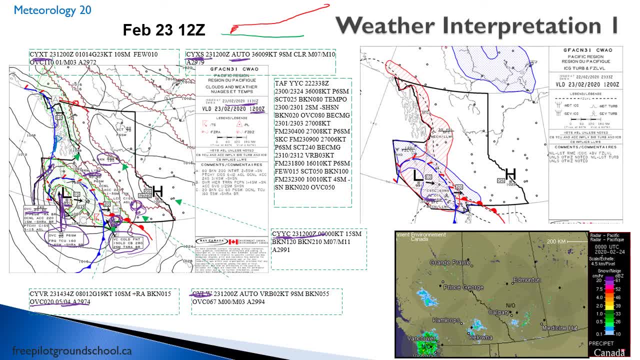 so that's going to be right here. this area moderate turbulence and occasional severe turbulence, and that's caused by that strong wind associated with that low. okay, so we have, and then up here we have mixed icing from the freezing level to top the 12 000. 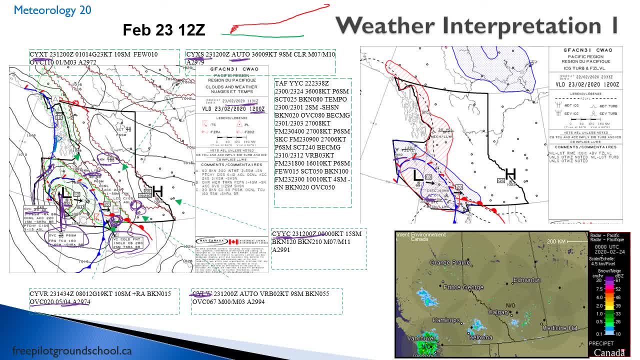 feet. so if you're flying ifr and you had to get on top, you want to get out of the icing, you have to get to 12 000 feet. so that should kind of stick out in your mind that you need an airplane that's going to perform and get to 12 000 feet in icing conditions. so you're flying around, let's say you're. 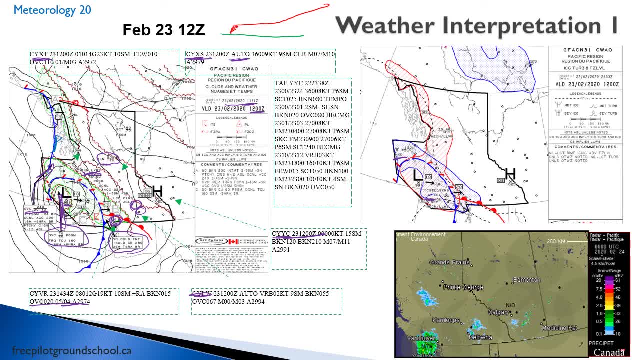 at 8 000 feet to get to 12 000. well, you do need oxygen on board. that airplane might not climb to 12 1, even climb to 12 000 feet with ice on it. so if you're flying in this weather, not only are your. 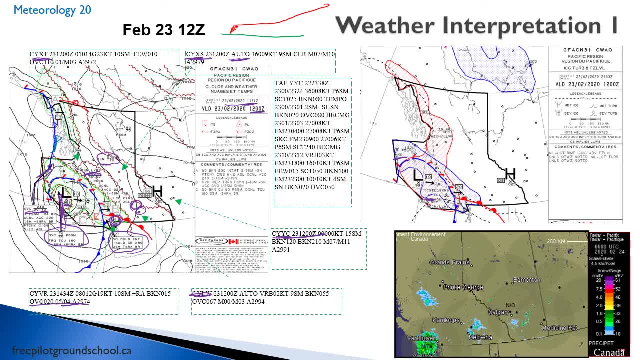 own capabilities, uh, going to be tested, but you also need to consider what kind of aircraft you have. so, for me, if i was uh flying this weather and you want at least a, a good turbo prop, uh, let's just say like a beach king air or something like that that i know is going to, it's pressurized. 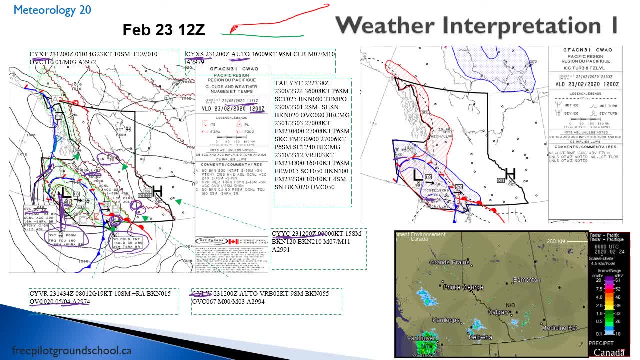 to get out of the icing above 12 000 feet. i don't want to get stuck in the mountains being unable to climb, unable to make an altitude because of the icing condition. so you, you also have to think about what kind of equipment that you're applying. if we look at the bottom here, here's this, here now. 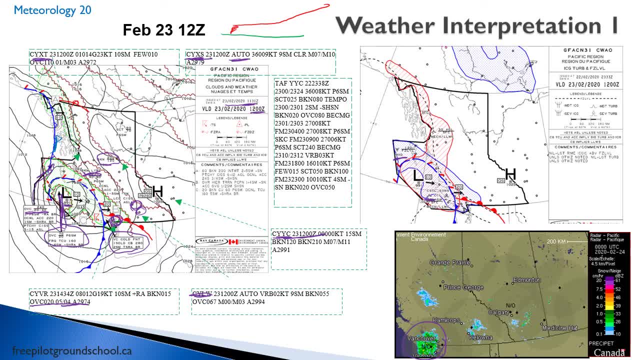 this weather shows up on the radar. so we have uh. that corresponds with about 30 dbz. uh, that is the rate of return. that's. that's a pretty strong return. uh, 30 dbz- a lot, um, and that's associated with all that uh precipitation here, that you see the heavy rain in vancouver. so that concludes uh.